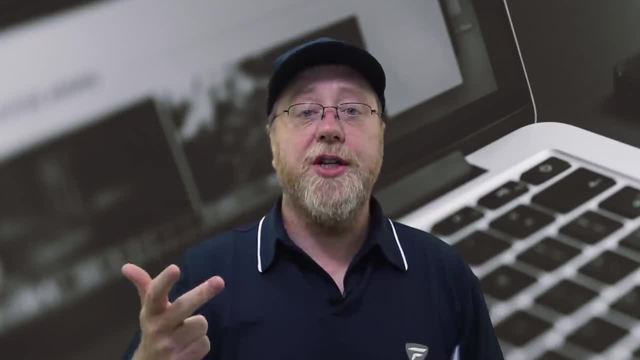 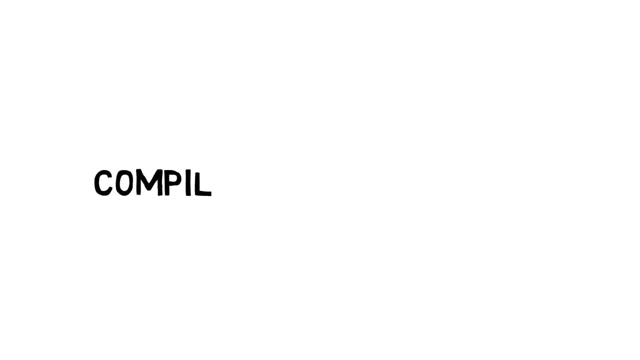 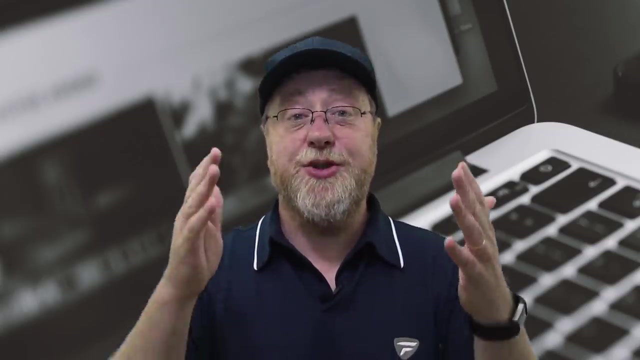 does it have static typing, does it use object orientation, does it have a garbage collector and does it offer concurrency? Okay, so the first thing we need to look at is if the program is compiled or interpreted. What does that mean? well, an interpreted program: you basically get a script. 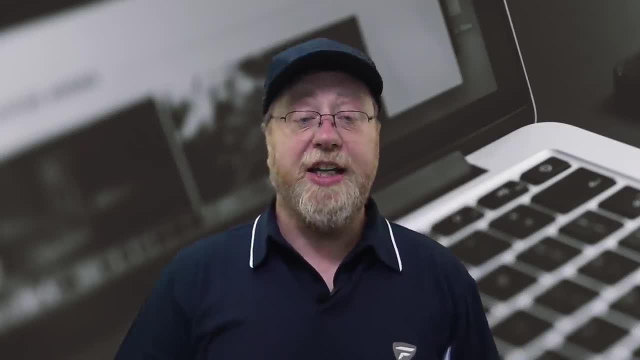 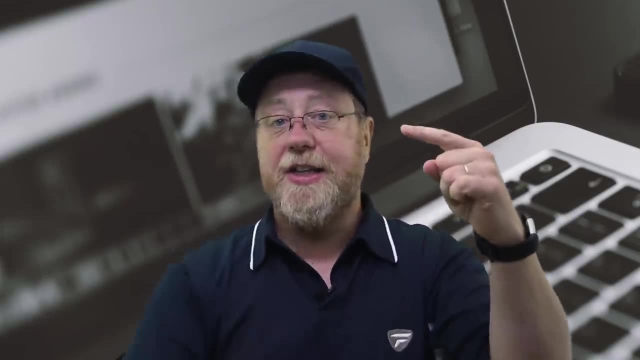 that's a text file that you've typed in and then you just run it. you say, run this script using using the language, and it starts looking at it one line at a time, doesn't look ahead to see what's at the bottom, and it just keeps going until maybe there's an error in the program and there it just. 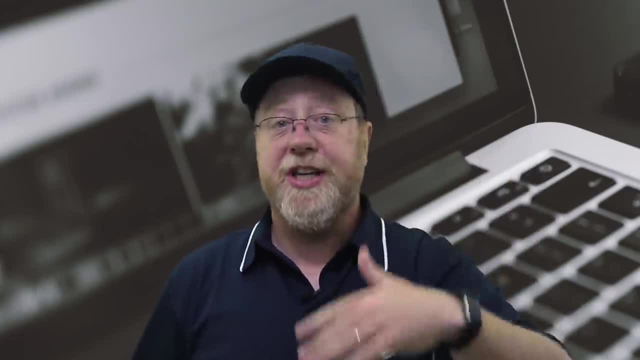 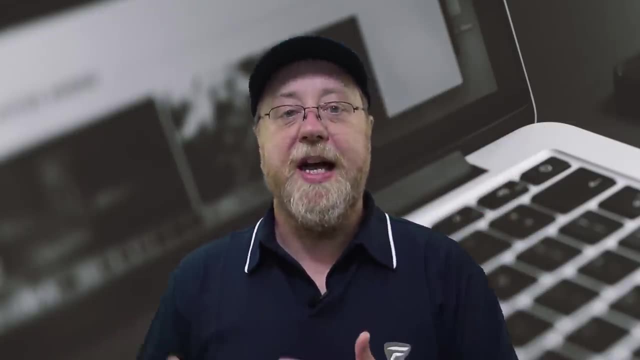 stops because it's just got to that point, or it runs successfully and just keeps on going. but every time it runs it's actually interpreting that line again and there are technologies to speed that process up. but in general what happens is it goes one line at a time. if it jumps somewhere, 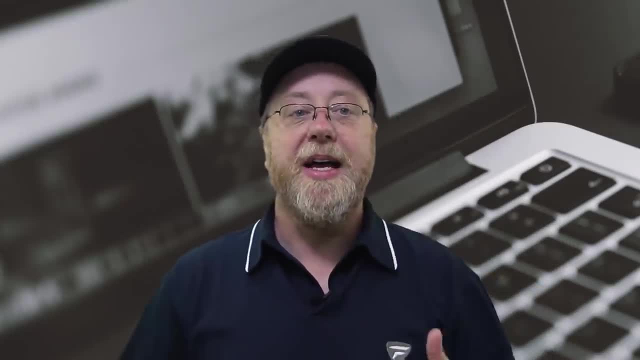 else it goes there in the code and it just looks at these lines, one line at a time, dynamically, interpreting it as it goes. now a compiled language is a bit different. with a compiled language, first of all you run it through a compiler, which means you take your program, which is written in a text. 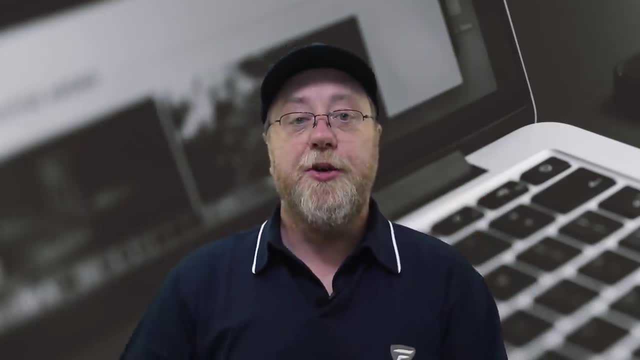 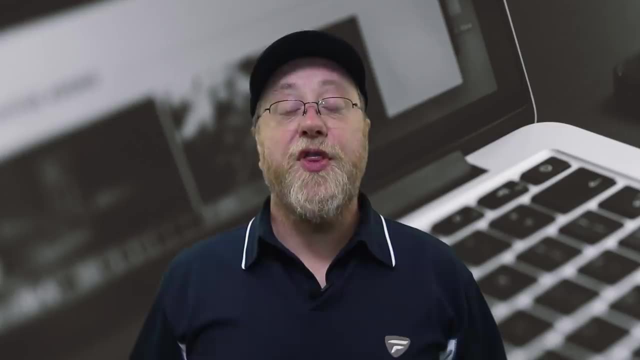 editor or in some kind of ide, and then you compile it to produce a binary and executable for the platform, whether that's windows or linux or mac os. there is a third variation, which is whether it's intermediate code. way back when, when they were porting pascal compilers from one mainframe to another mainframe, they found that 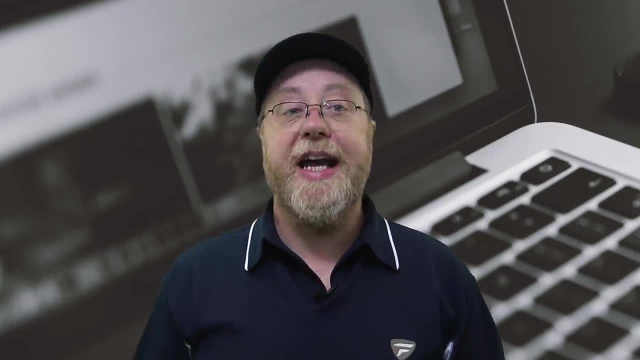 actually this could be quite a difficult task. so they came up with the idea of a pascal compiler that produced p code for porting, and this intermediate language was actually used on every machine and on the different system you were porting it to. you just had to create an. 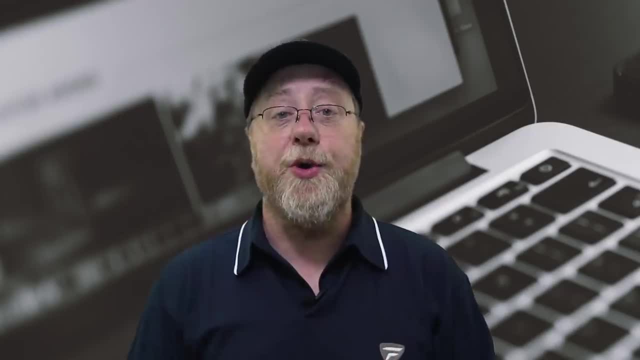 interpreter or some kind of virtual machine that would run that p code and that made the porting of the compiler from one system to another system much, much easier. and in fact we still use this idea today when you come to things like java and c sharp. so for java you. 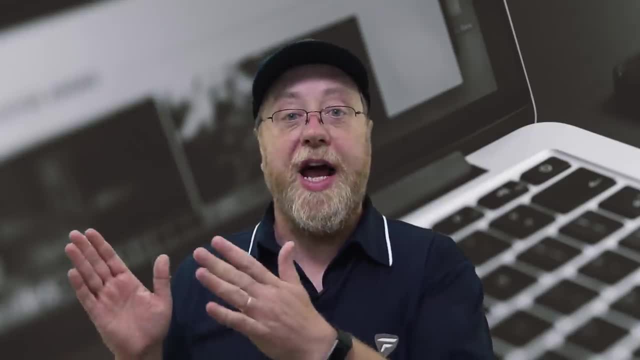 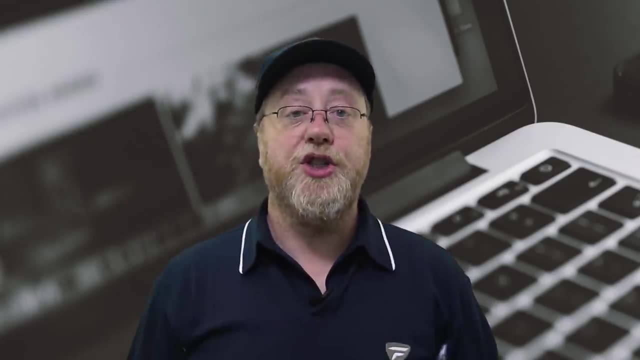 have the byte code which runs on a java virtual machine, and that's what happens today on android smartphones. apps are compiled to java byte code. the byte codes then run on a java virtual machine and then, of course, you've got c sharp which runs on the clr, which is the runtime environment for 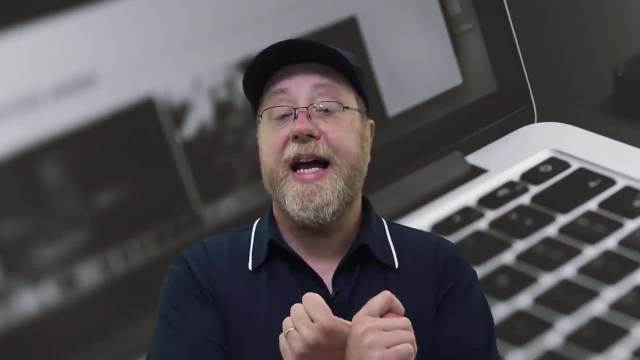 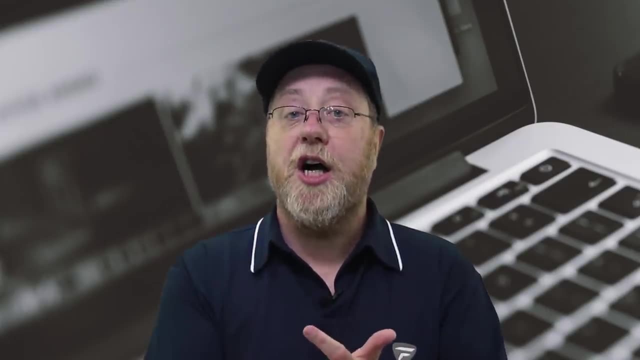 the dot net framework. so you've got interpreted, which would be a language like python. you've got compiled, which would be something like c, and then you've got intermediate code, which would be something like java with its byte code. let's talk about typing for a moment now in some languages, if you want to assign five to a variable. 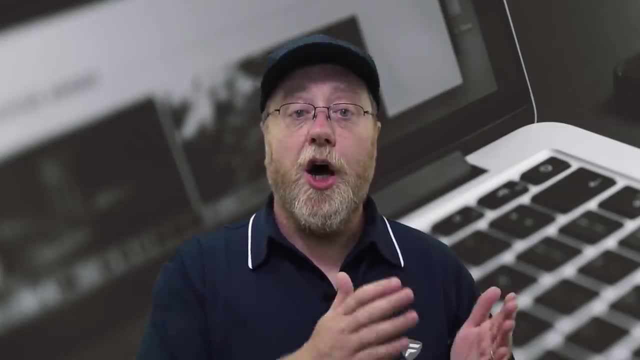 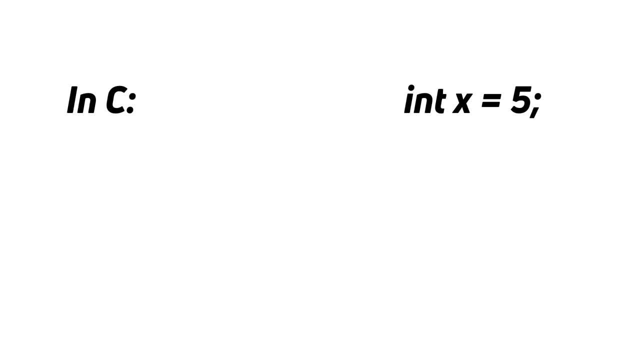 you have to tell the compiler that that variable can take a whole number, so we call those integers. so in c you might say: int x is equal to five and that tells the compiler that it's an integer, can go into x, and five of course is an integer. but in other languages like python, what you actually get 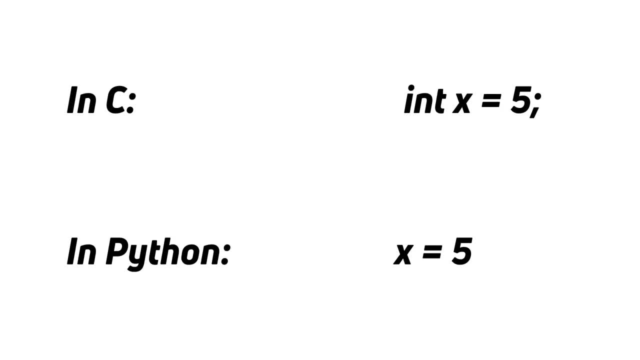 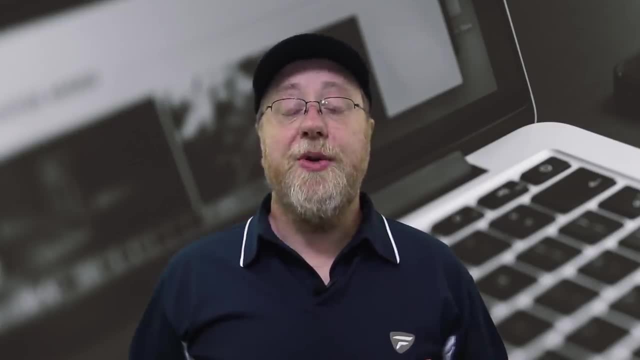 is that you can just say x is equal to five and the interpreter says: well, five's a number. so we're going to say that, therefore, x can hold integers, and then you also get strong typing and weak typing, which means that in some languages you can swap between different types very easily. so if 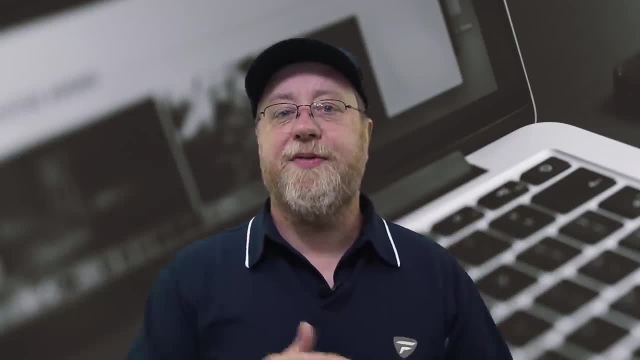 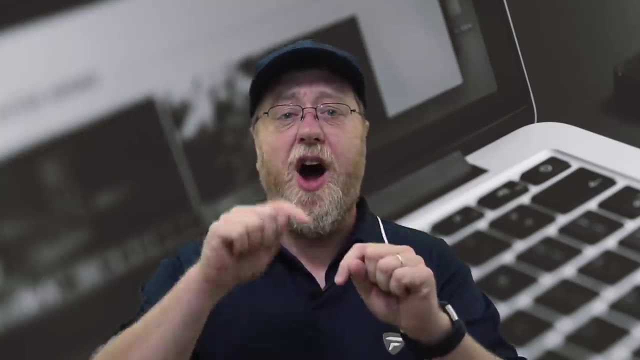 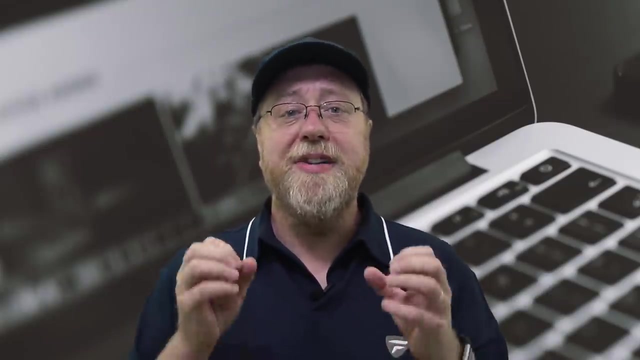 you've got a long, which is a way of storing a big number, you can maybe transfer that to an integer, which is a shorter number, without much effort. other languages make you really really kind of say: integer into an along and so on. so strongly typed languages really make you say: 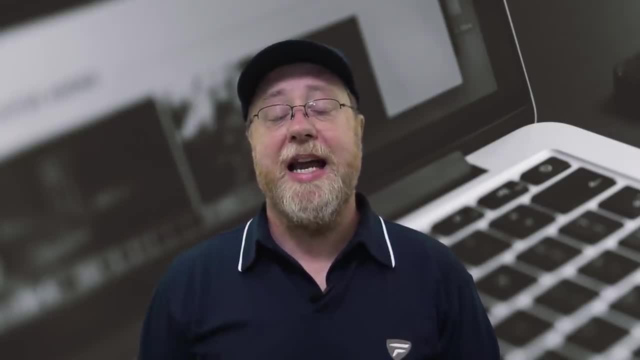 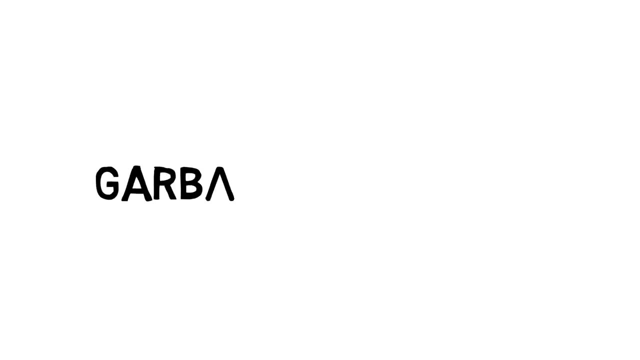 what you're intending to do and weaker typed typed languages. let you just kind of do it in a more blase fashion and we just kind of hope it all works out at the end. now another thing to consider is garbage collection. when you have a complex program, you're probably dynamically 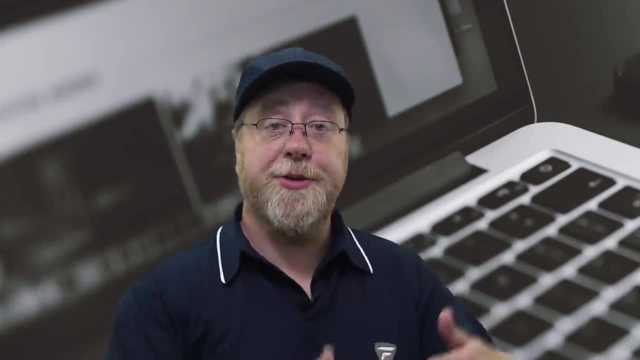 allocating memory. you want a space for a string, you want a space for a table, you want to do something with a matrix and you kind of allocate that memory. you want to have to have memory to speak to, meaning that if you're going to send something to another variable which is a long, stuck wheel, various. 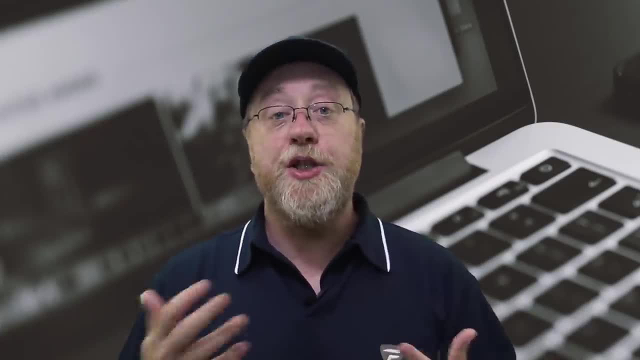 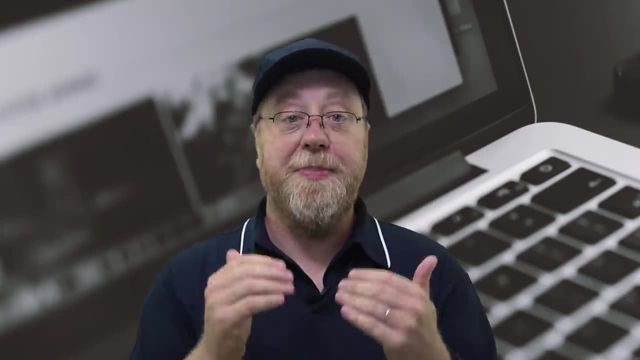 memory as you are running the program. now, once you finish with that variable, once you finish with that string, once you finish with that table, what happens to that memory? well, in some systems you have to explicitly say: i want to free that memory, that memory is no longer being used. other systems: 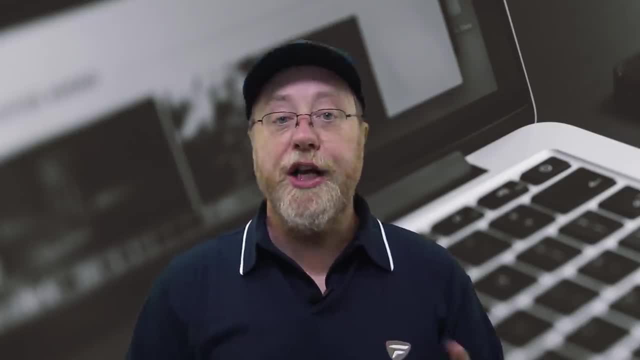 which have a garbage collector, they work out that you're no longer using that variable. there's no links to it, kind of dynamically in the program as it's going along. there's no reference counts. that's the kind of the term that's used and it will then go through the list of things that are. 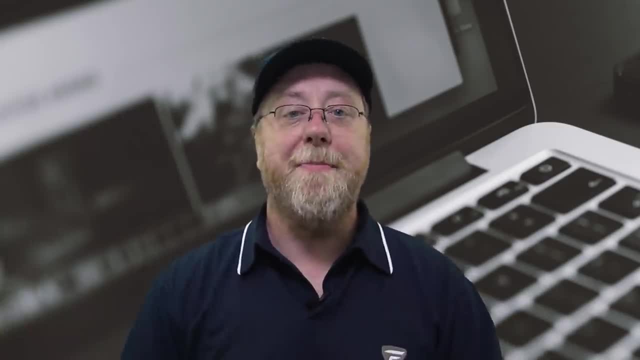 no longer used and it does garbage collection, kind of freeing up all the memory as it goes along now. garbage collection is great in the sense that you don't get memory leaks, because the compiler and the program kind of get the idea of freeing up the memory you don't need. 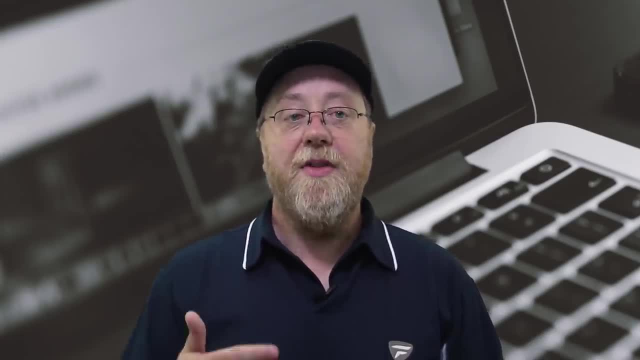 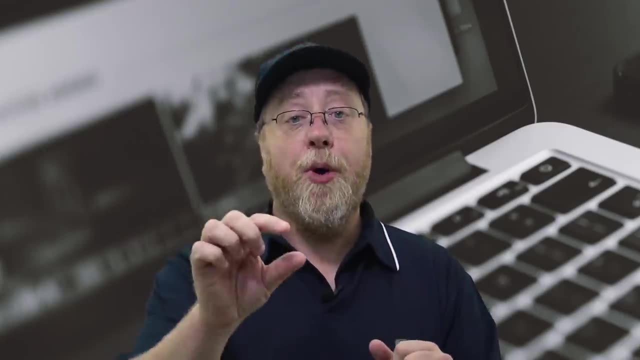 but there can be an overhead because you can be running something and then suddenly the garbage collector says: oh, i'm going to run now and just as you were about to, you know- do something that was time critical. then there's a pause because the garbage collectors decided to start tiling up the memory. so there are arguments for and against whether you want. 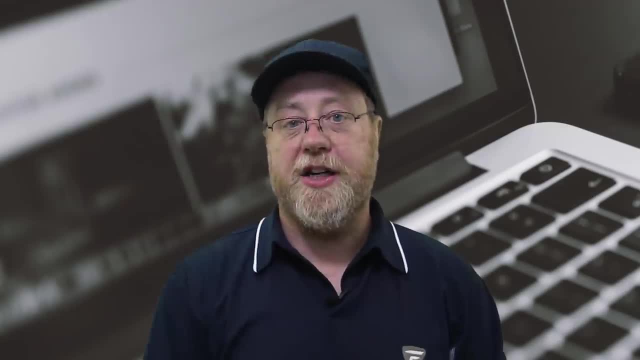 to have garbage collection. now, a language like c does not have garbage collection. you have to manually allocate and free up, deallocate any memory, and a language like java has a garbage collector so that when you're no longer using certain things, they will get removed from memory. 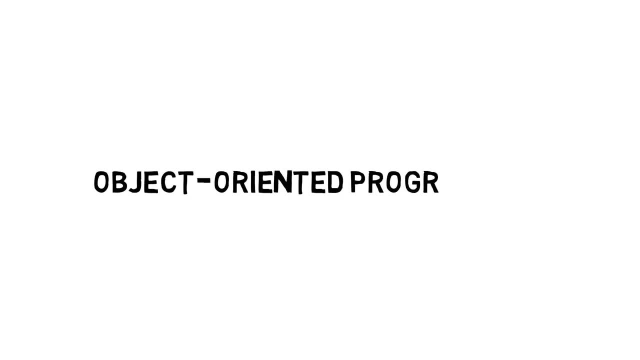 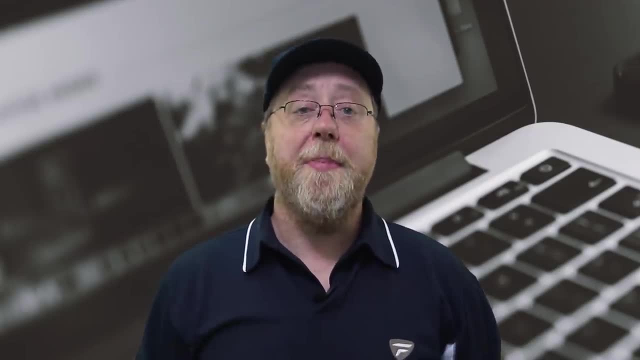 automatically. another important aspect of course of a program now is: is it object orientated? that basically means: can you create classes, can those classes be inherited, and so on. now, basically, the idea here is that you might say: i want to define a type of vehicle and then a type of. 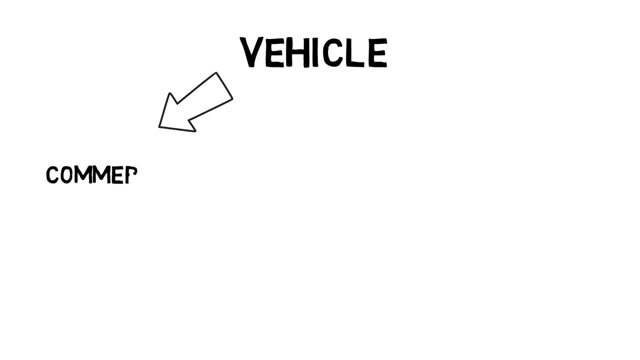 vehicle might be kind of commercial or might be kind of a family, and then under family you might say that it's a car, and under commercial you might say it's a truck, and then you might say it's a truck with so many wheels and so on and so on. so you can kind of build up this hierarchy of objects. 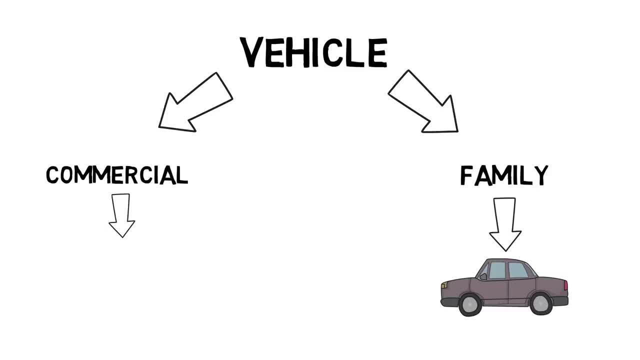 kind of the real world and they relate to each other. so their cars and trucks are both types of vehicle at the top level, but only car is a type of family vehicle and only truck is a type of commercial vehicle, and so on. now again, there are lots of pros and cons for object orientated versus 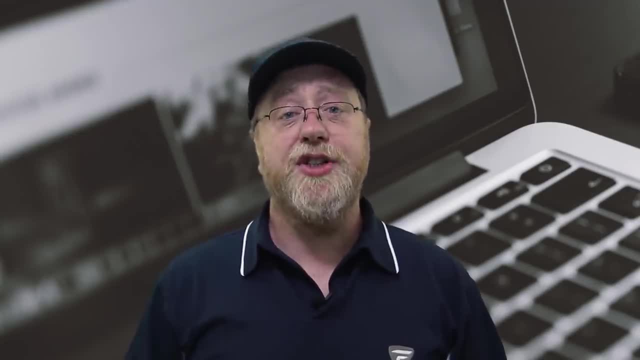 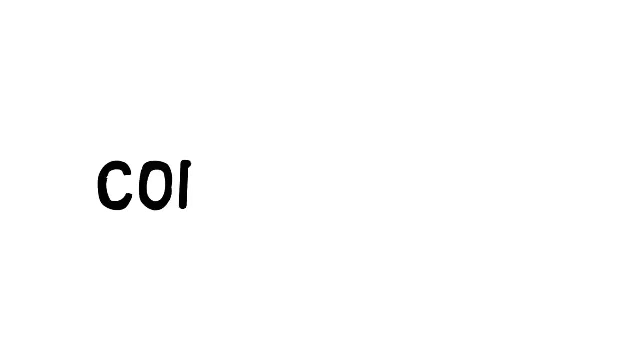 non-object orientated. certainly object orientated was very much in vogue. we've got things like c++, c, sharp, java, all object orientated languages. when you come to language like golang, then that has to be in a position of things like c, where it's not object orientated. and the final thing i want: